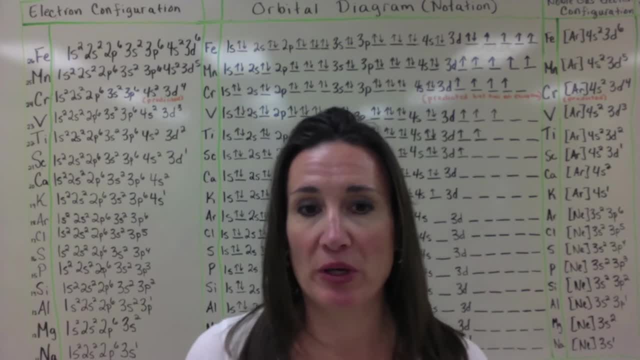 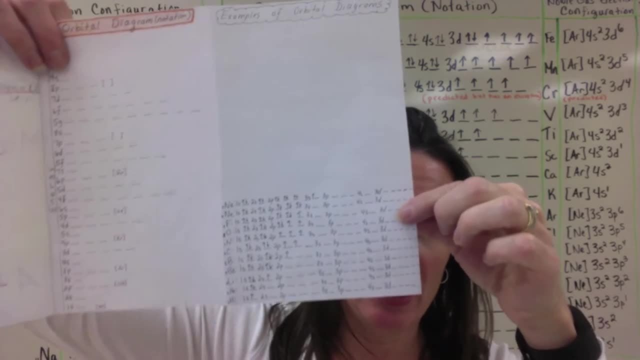 If you have a hard time including all these orbital diagrams in your foldable- the way it's built- you can add an addendum page. So on this page here where you have a blank orbital diagram, you can leave it blank and then tape a half a sheet of piece of computer. 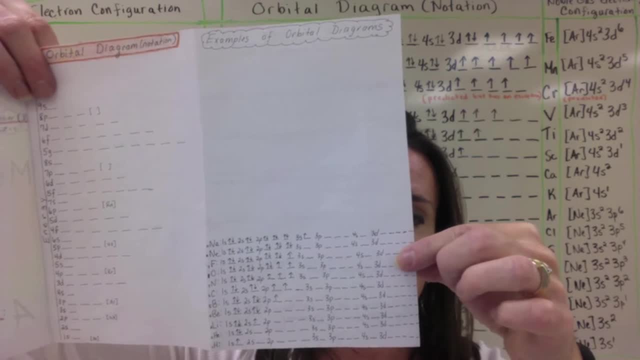 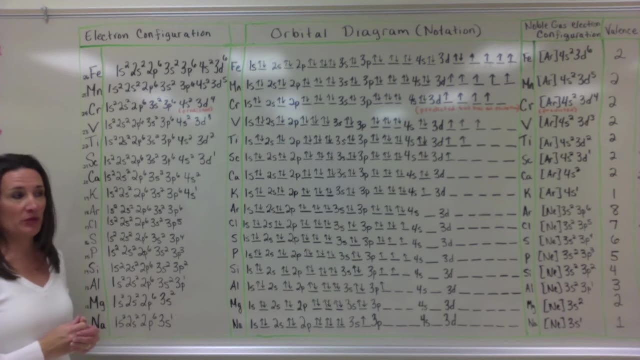 paper that you can then do. hydrogen all the way to iron's orbital diagram. Here are those electron configurations for sodium all the way to iron Orbital diagrams for those elements, the noble gas configuration for those elements and the valence that those elements have. 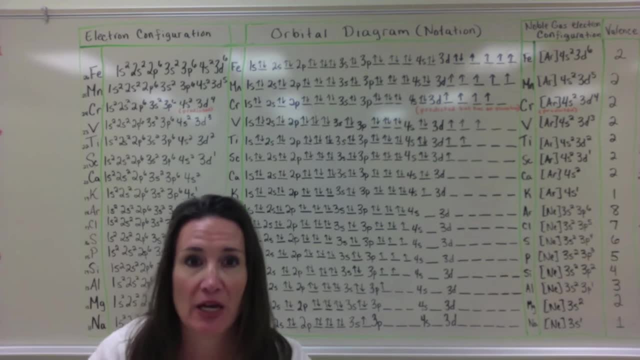 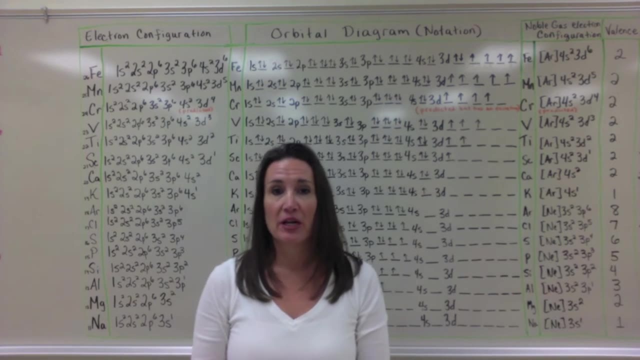 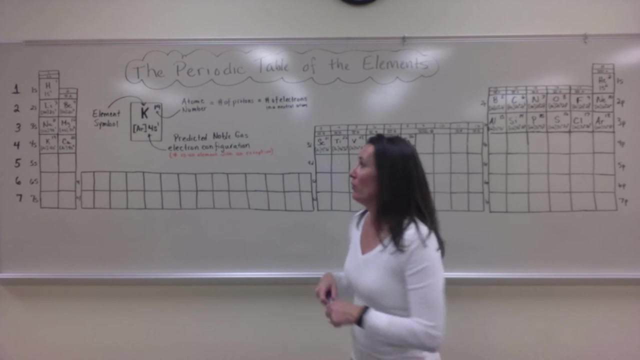 What you do next is take all those noble gas configurations and grab your gigantic periodic table that we made before, and we're going to add those into each box so that you can see that there's a pattern that you can use to predict the configuration of any element on the entire periodic table. Here's what your periodic table looks like. 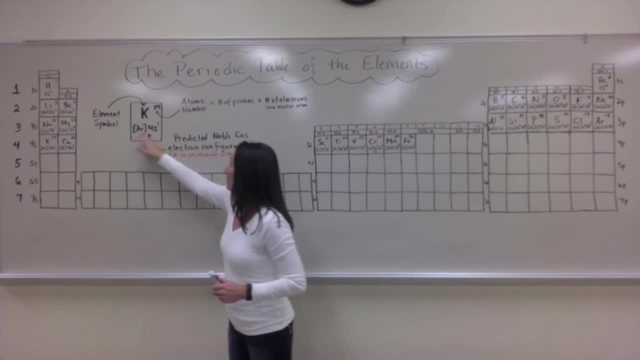 What you'll need to do next is fill in the electron configuration underneath the element symbol for the elements that we've already done- hydrogen all the way to iron- and that will get you to here. After that, you have your have to use an orbital diagram, or maybe you can start to predict the configurations of the rest. 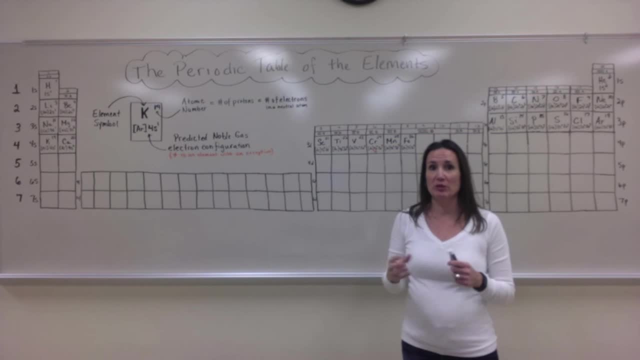 of the elements, using that off-ball principle, which means building up or construction, and what you'll need to do also is label those gaps with some helpful hints as to which orbital you're filling. For example, f will be 4f and 5f, d will be 3,, 4,, 5, and 60, and then p will go back to being